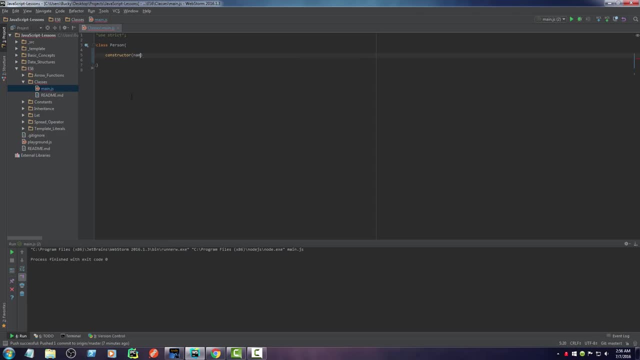 and you just call it constructor. Easy enough. So now, any values or attributes that you want to initially set, you just pass in So name, age, weight, Boom, roasted. Now, of course, you want to make these attributes, You want to make these attributes specific to this object. So, thankfully, we can use the 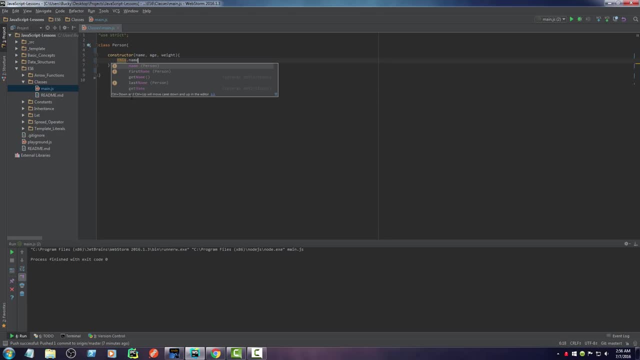 keyword this. Now, whenever we hit something like this name equals name, then what this means is whatever name we passed in is equal to this object's name And, of course, what this allows is for you to be able to create multiple different people, and they each have. 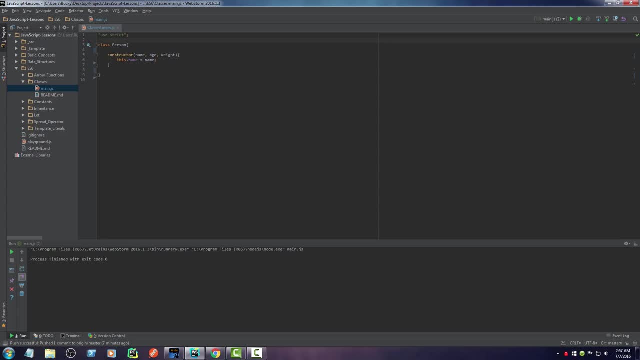 their own name. So Bucky can have his name, We can create another person called Sally, She could have her name, so on and so forth. So this would be something like this age equals age and this weight equals weight. So later on I'm going to show you guys how to create multiple objects and they each have. 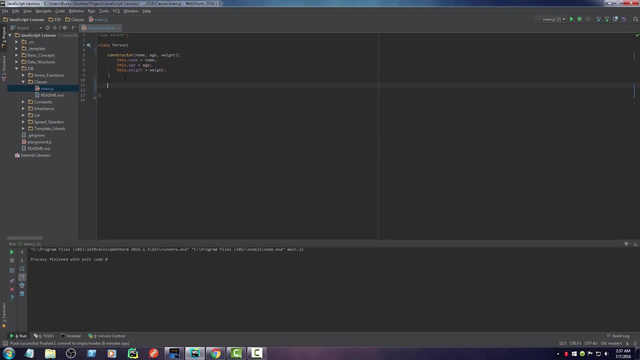 their own set of properties. And that brings me to another point. People ask me a lot: When do you use classes and when do you just create a bunch of, you know, standalone functions? You're going to create a class whenever you have a bit of code that you need to be able. 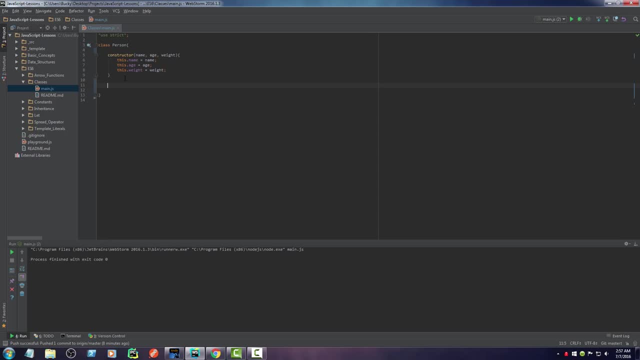 to use. You're going to create a class whenever you have a bit of code that you need to be self-aware. So I always have like helper functions, like to write a file, parse Jason, do whatever. Whenever I use those, they're pretty much just a little snippets of code. 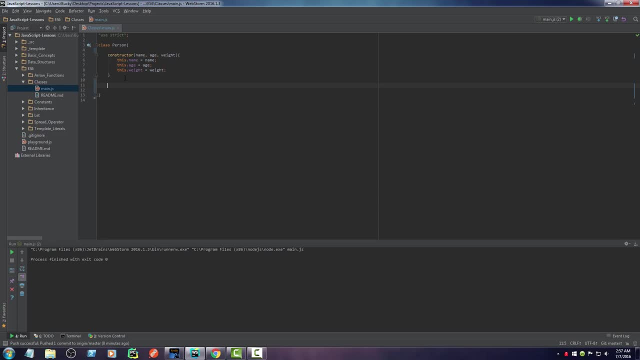 that run and then they're done. I don't need them to remember anything or do anything special. Now, whenever I create a person, object, then this person or this is a little bit of code. it's going to need to remember its name. It's going to need to remember its age. It's going 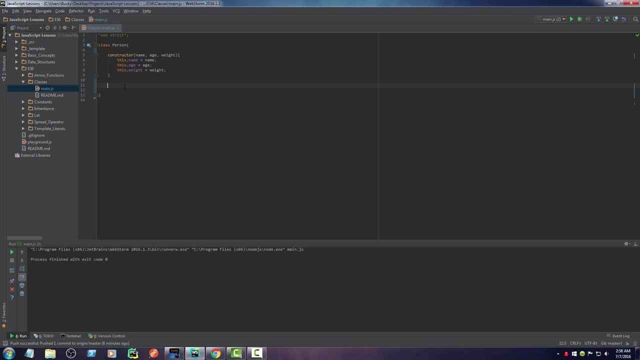 to have some bit of memory That it needs to be aware of. So that is when you write a class versus just a bunch of functions. Whenever you need a bit of code to be self-aware or remember something, stick it inside a class. 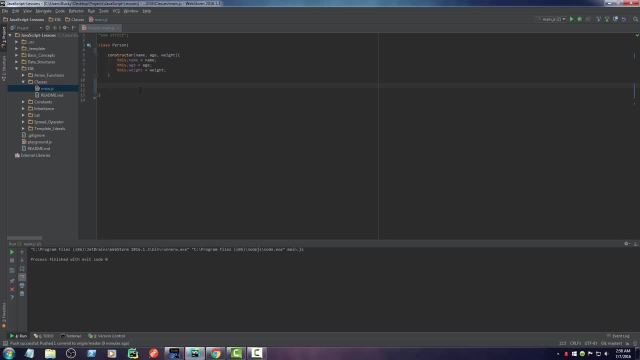 Also, if you just have a bunch of similar code and you want to group it and make it a class. but there you go, All right. So instead of just making constructor in here, you can also have methods. So I'll say display weights, and this is just a method that displays the